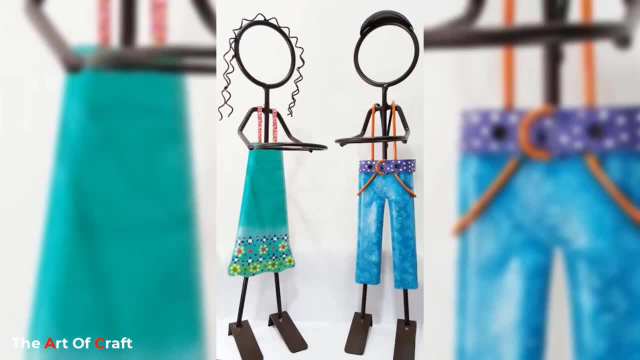 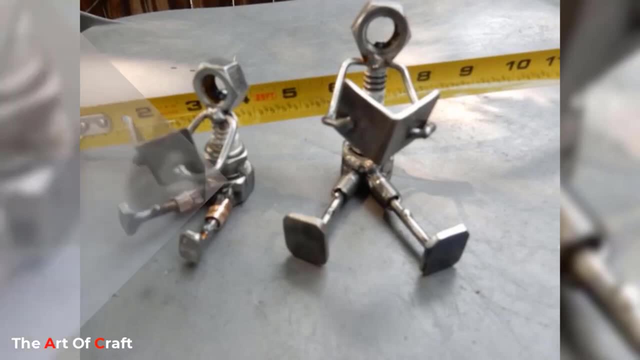 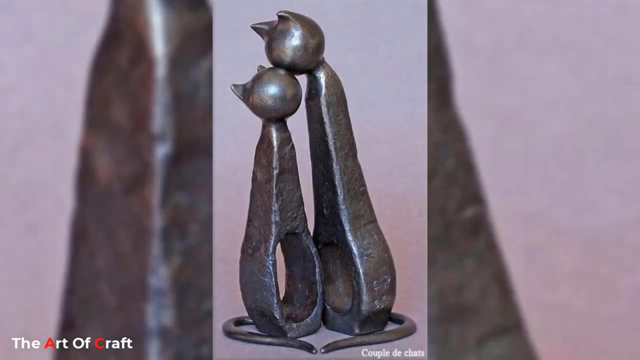 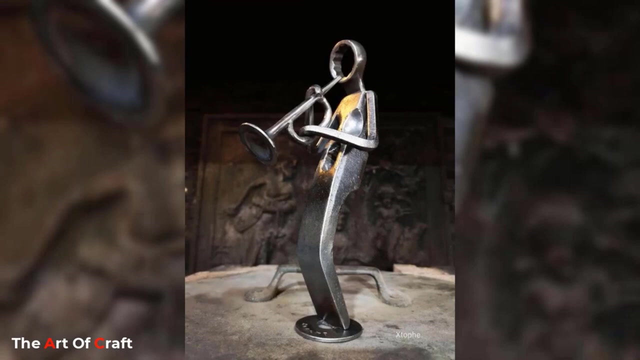 What is scrap metal art? Scrap metal art is a unique and fascinating form of expression that transforms discarded metal into stunning works of art, From sculptures to garden decor. there is no limit to the creativity that can be unleashed from this medium, Whether you are an aspirant or an artist, scrap metal art is a unique and fascinating form of expression that transforms discarded metal into stunning works of art. 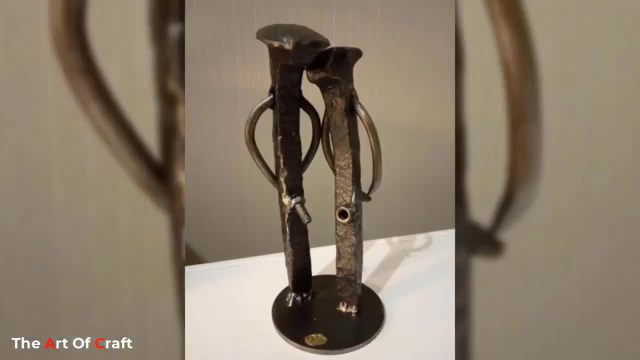 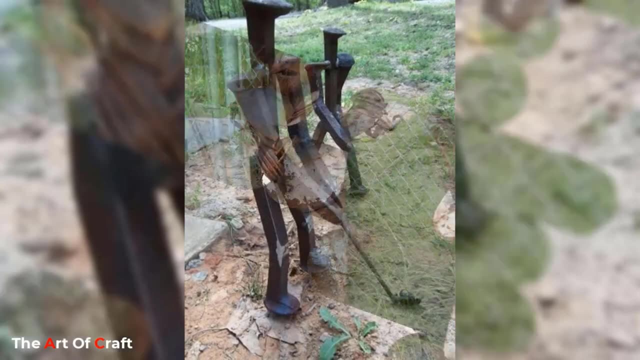 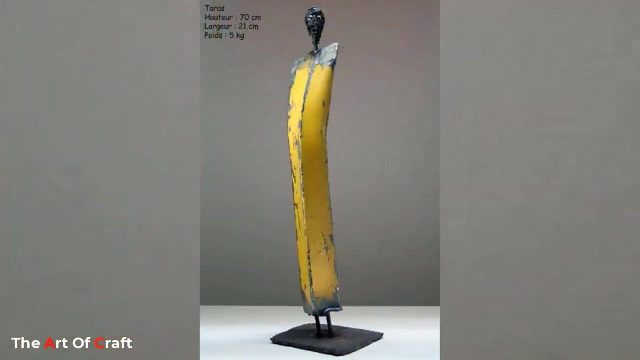 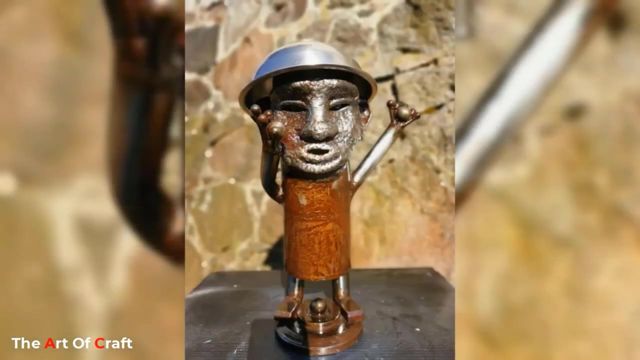 Whether you are an artist, DIY enthusiast or just looking for a new hobby, here's a beginner's guide to get started with making scrap metal art. Today, scrap metal art has evolved into a vibrant and diverse field, with artists working in a variety of styles and mediums to create work that range from abstract sculptures to functional objects such as furniture. 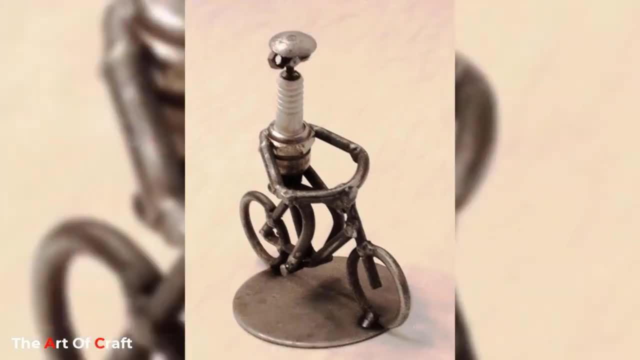 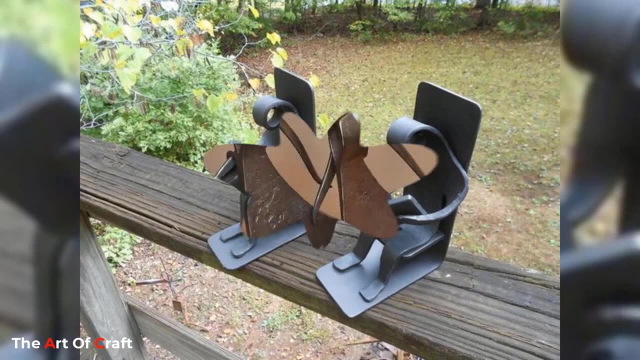 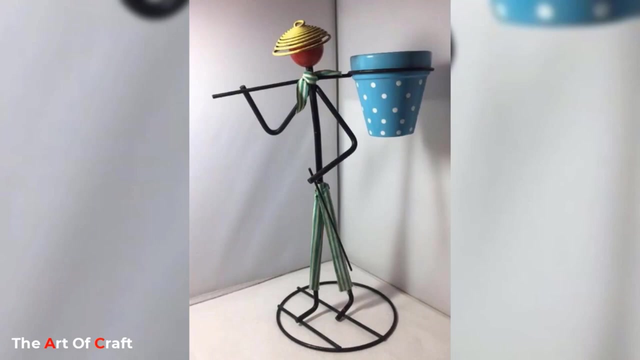 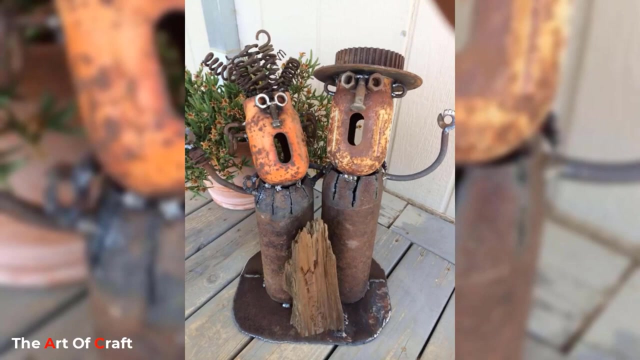 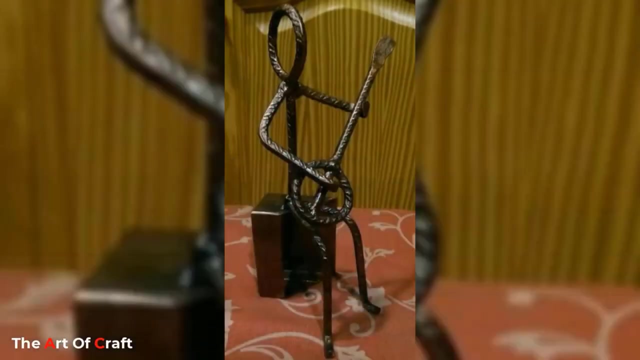 and lighting fixtures. The use of discarded metal scraps in art continues to be an important way for artists to reflect on the impact of industrialization, technology and the environment and to create work that are both aesthetically pleasing and environmentally sustainable. Steps to creating scrap metal art. Step one: gather your tools and materials. 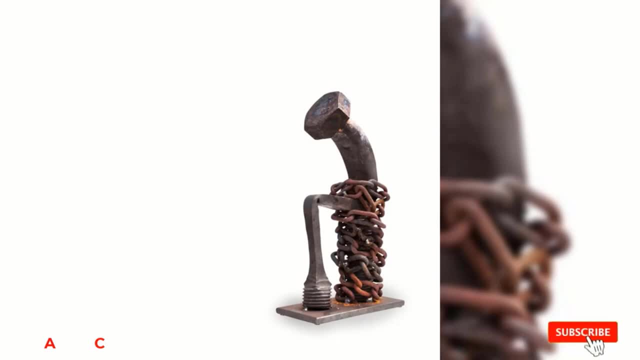 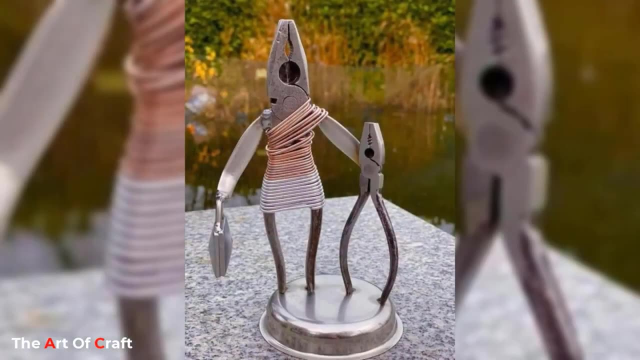 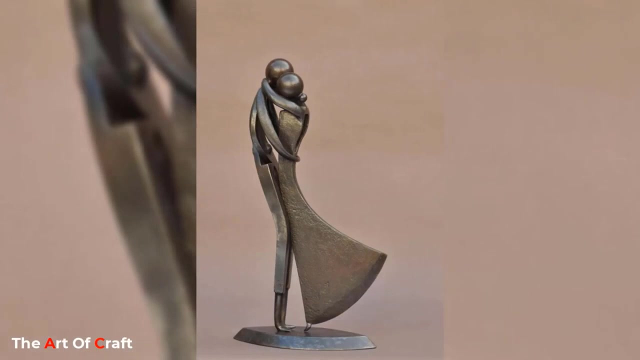 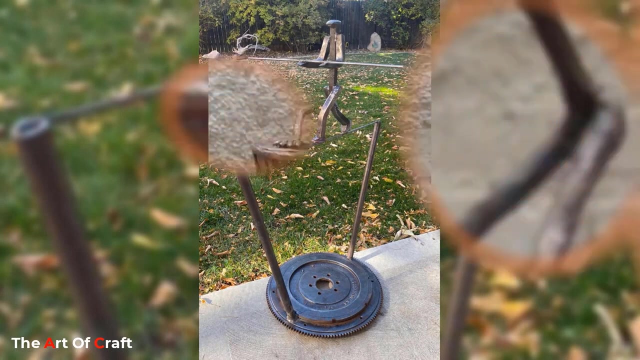 The first step in creating scrap metal art is to gather the right tools and materials. You'll need a variety of metal scraps, such as steel, aluminium or copper, and a range of tools, including metal cutting saws, pliers and welding equipment. If you are just starting out, you may want to. 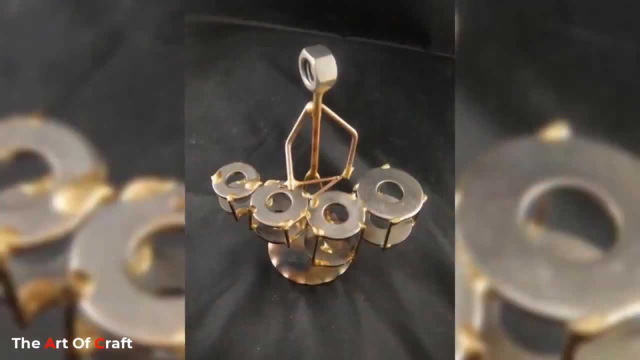 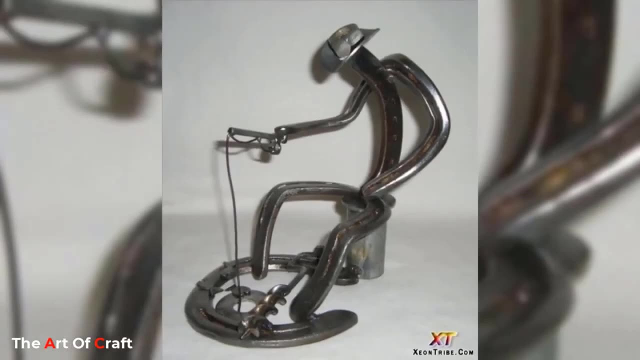 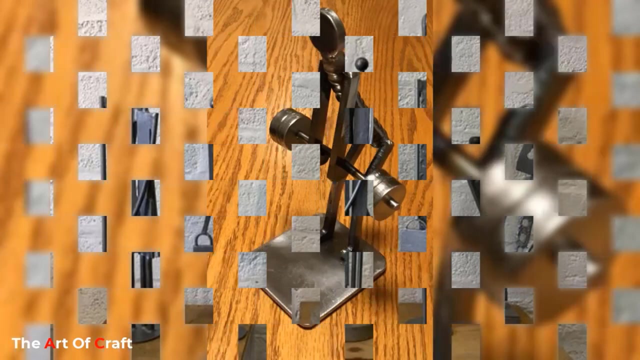 invest in some basic tools such as metal snips, pliers and a hammer to get started. Step two: Plan your piece. Before you start creating your scrap metal art, it is important to have a clear LISA parallel scale idea. Pause when needed a claws and a chair. Does this make our work easy and user-friendly? 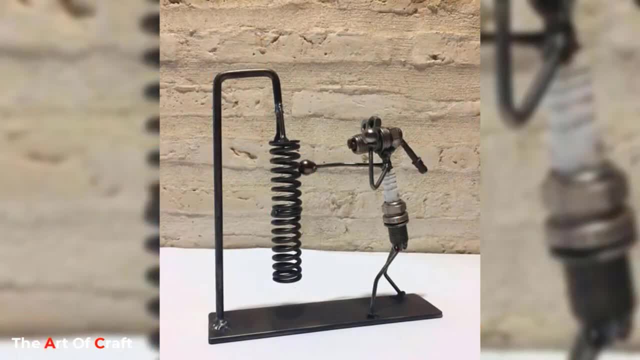 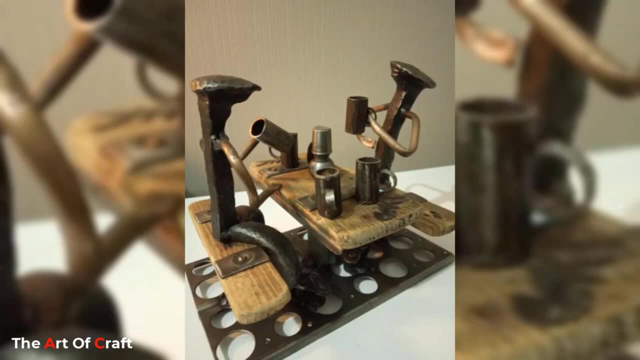 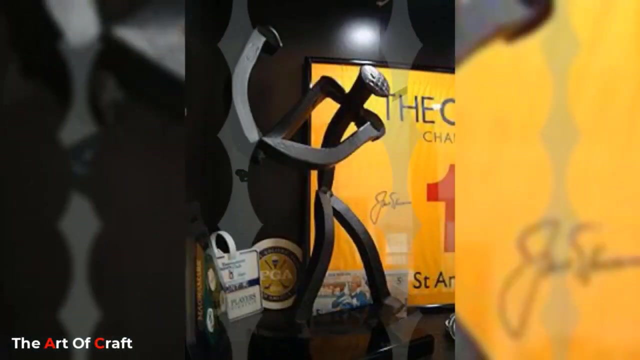 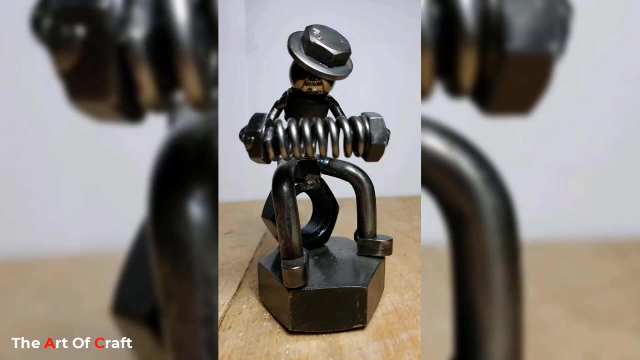 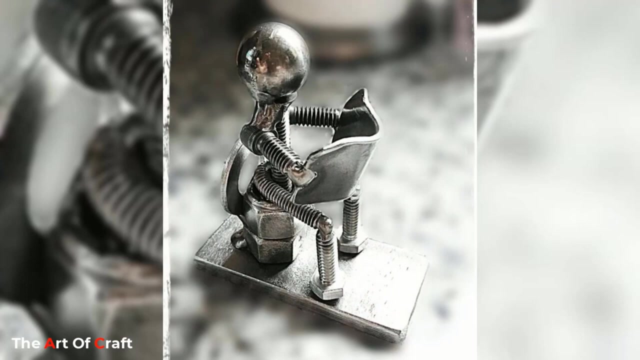 idea of what you want to make. consider the size and shape of your piece, as well as the type of metal you want to use. you may also want to consider the overall design and theme of your piece, as well as any special techniques or tools you may need. step 3: cut and shape your metal. once you have a clear plan in mind, it is 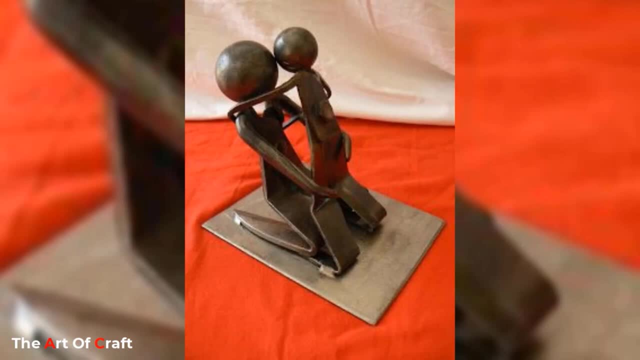 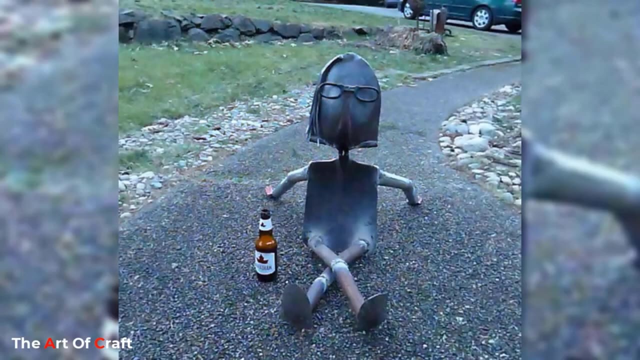 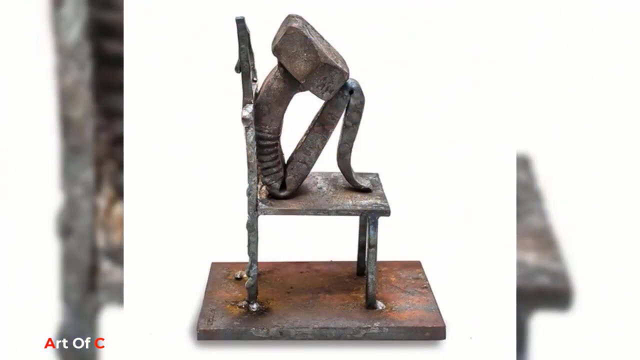 time to start cutting and shaping your metal. start by cutting your metal scraps into the shapes and sizes you need for your piece. you can use metal cutting saws or snips to achieve this desired shape. now you can cut and shape your metal to the desired shape. 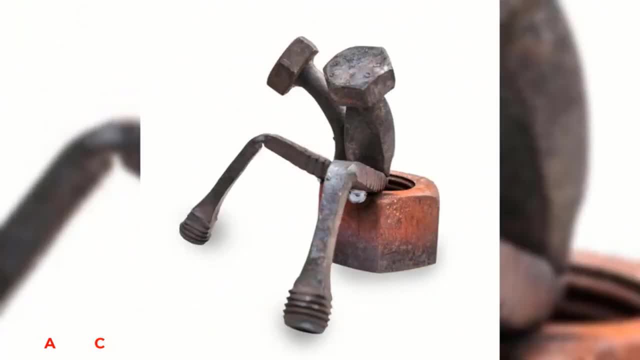 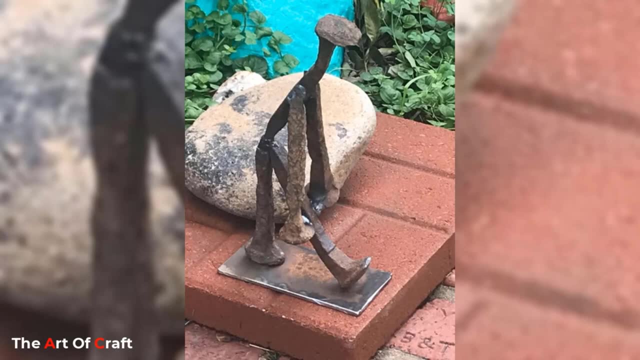 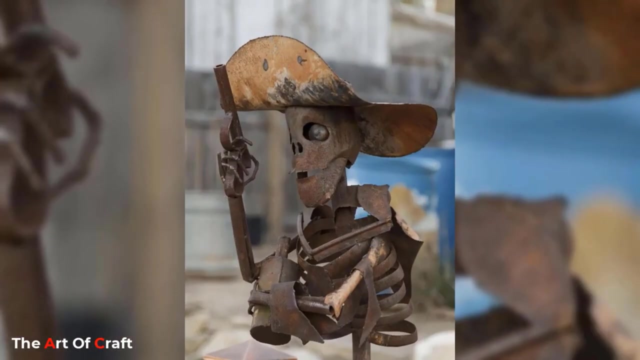 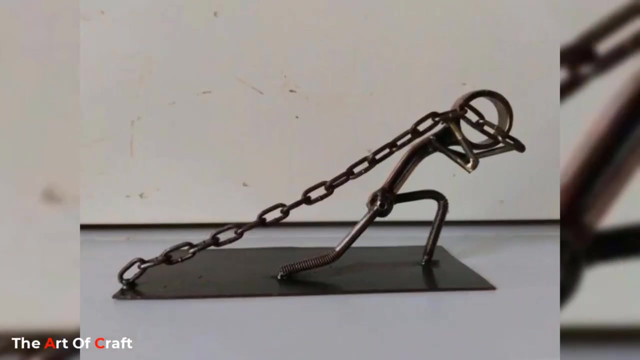 next, use pliers and other tools to bend and shape the metal as needed. check out these articles for other metal cutting tips. step 4: weld the pieces together. when your metal pieces are cut and shaped, it is time to start welding them together. this is an important step in creating a strong, stable structure. 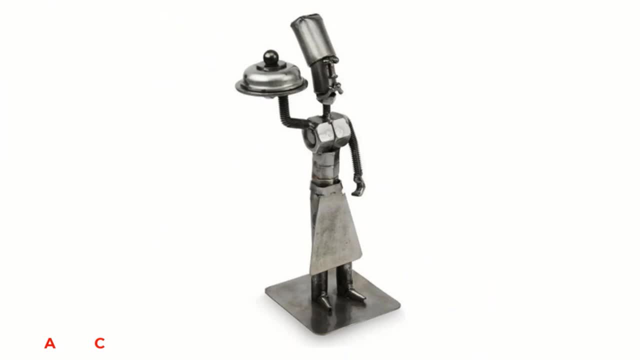 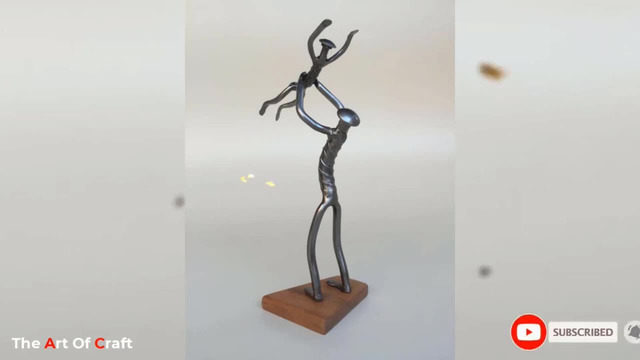 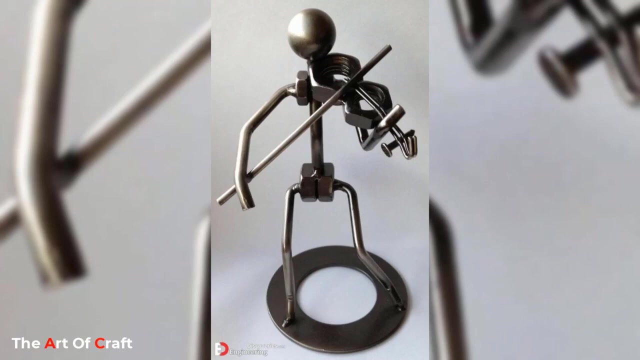 for your scrap metal art piece. If you are new to welding, it is important to start with a basic welding technique, such as MIG welding, and gradually work your way up to more advanced techniques. Step 5. Finish and protect your piece. The final 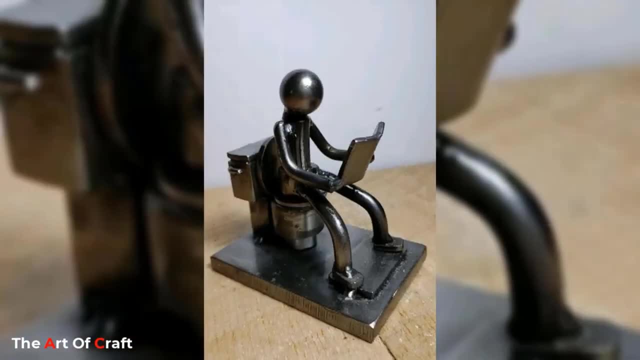 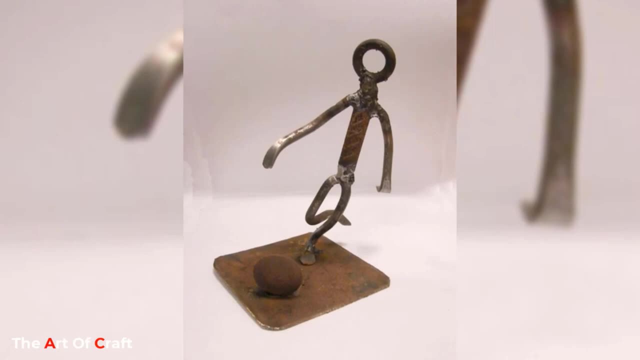 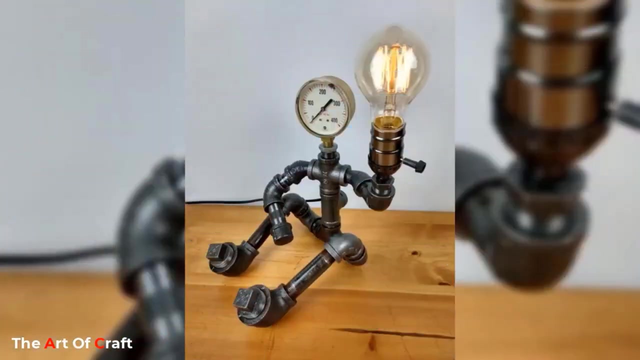 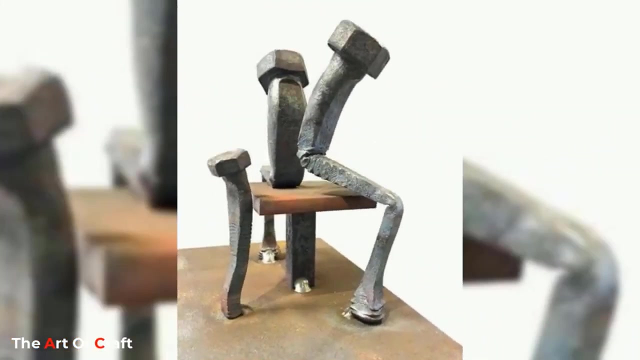 step in creating scrap metal art is to finish and protect your piece. You may want to add a coat of paint or primer to protect your metal from rust and other forms of corrosion. You may also want to consider adding a clear coat of protective finish, such as clear polyurethane, or ensure that your piece 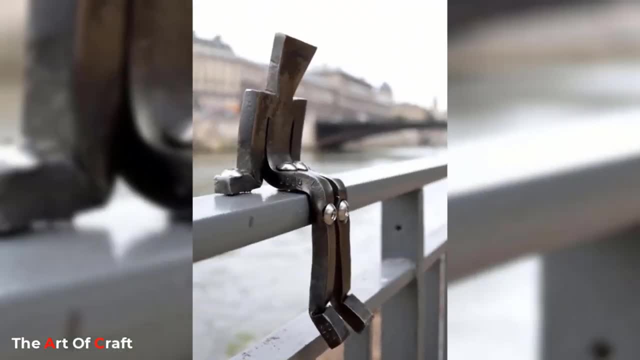 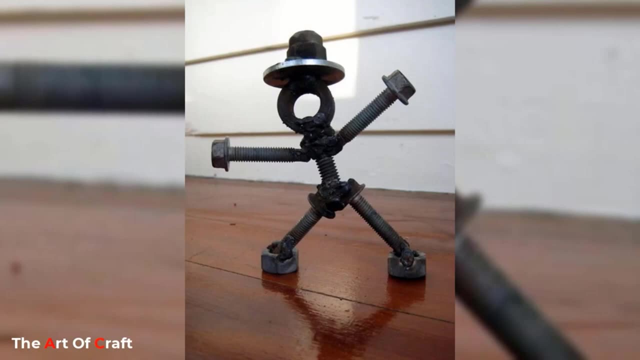 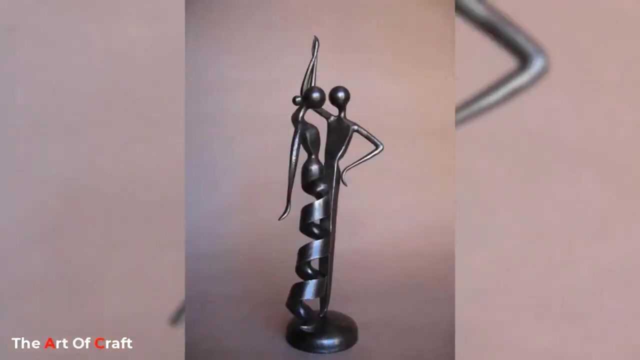 lasts for years to come. Well, I hope you have enjoyed this video. If you have any questions, feel free to ask me in the comments. Now to find material for scrap metal art. Material for scrap metal art can be found in many places. Check out our guide to finding scrap metal for a more. 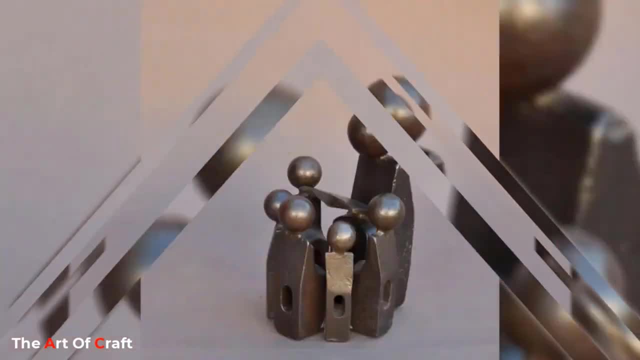 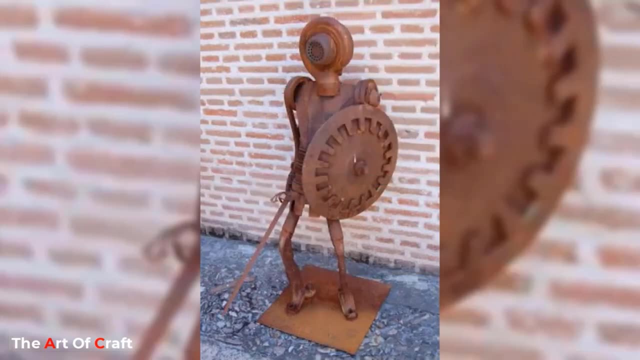 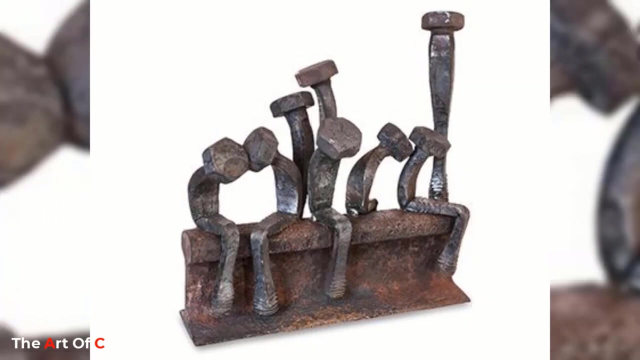 in-depth look. Metal can be found at the curb, on garbage land. Just remember you will be competing with scrappers. You can visit fab shops and machine shops and ask for their scraps and cut-offs, often called drops. They may not be free. 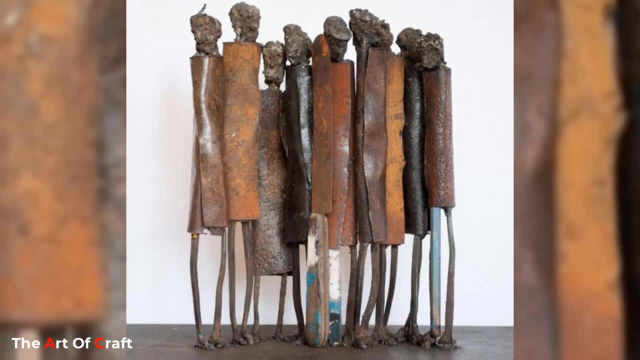 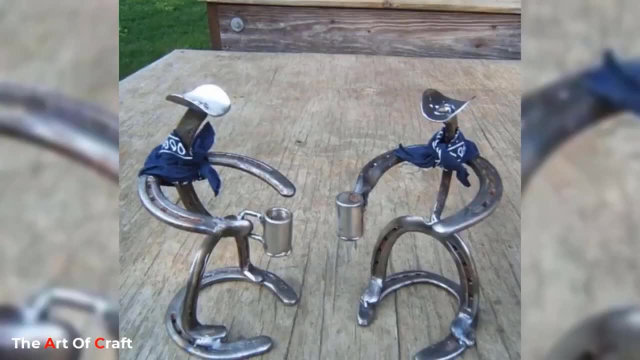 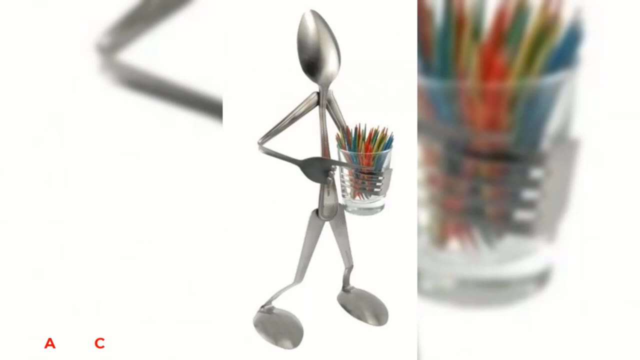 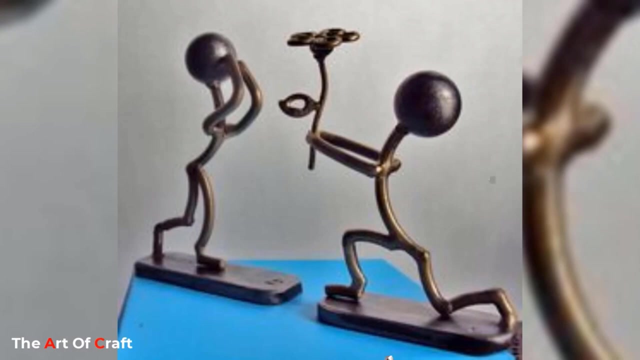 but they are often cheap. Garage sales can be a good source of metal if you think outside of the box and look for buckets of nuts, bolts and other assorted metal items. Swap meets are a great source of interesting pieces and parts. Think gears, light housings and springs. 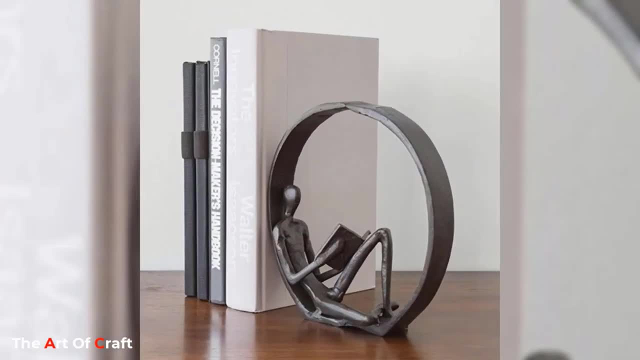 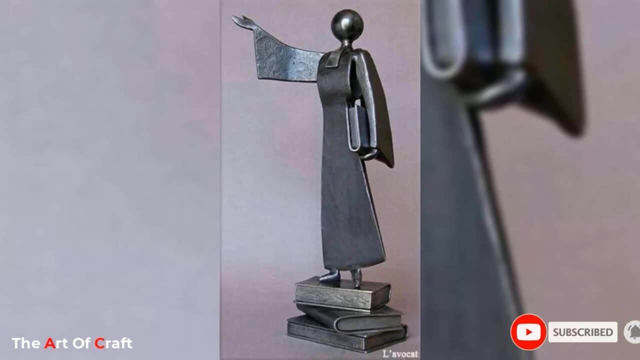 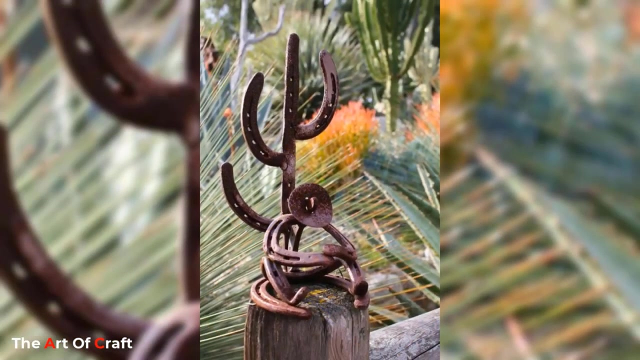 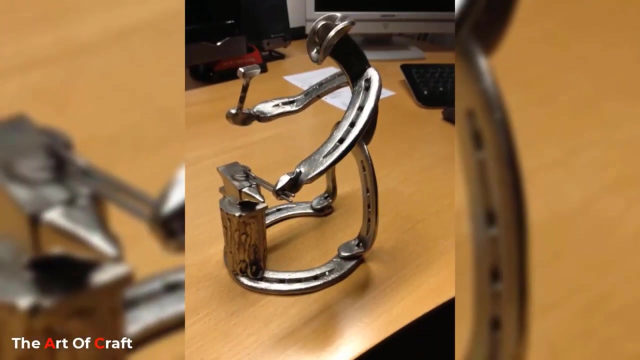 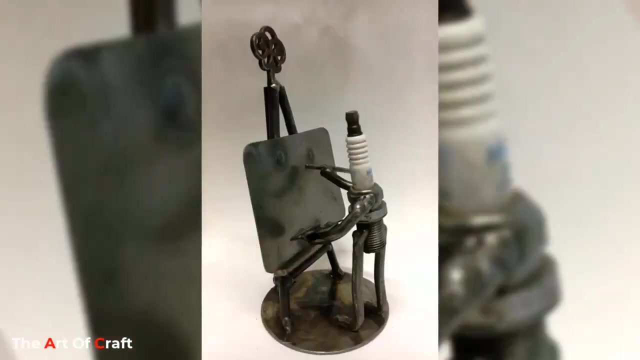 Second-hand stores often have very cheap silverware. You can also find deco lamps, cookware and other metal objects to use. Making scrap metal art is fun and a rewarding hobby that allows you to turn discarded materials into beautiful works of art. Whether you are a seasoned artist or a beginner, the key to success is to have a 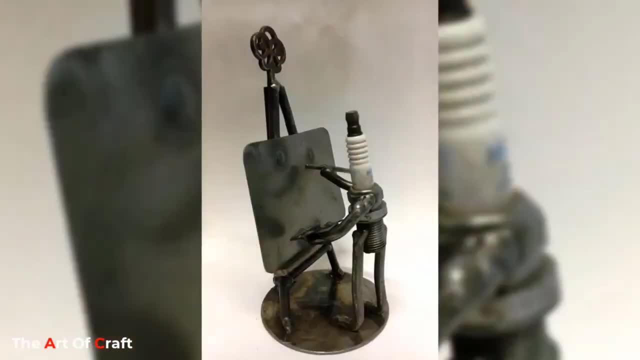 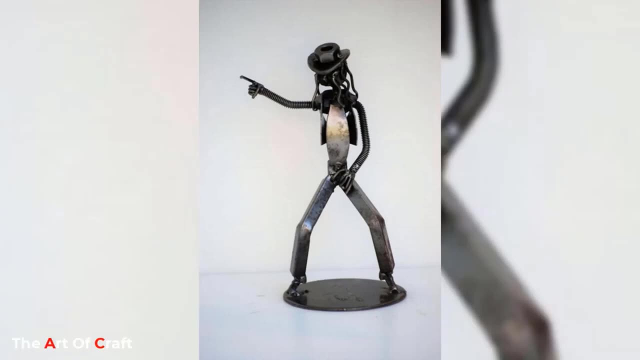 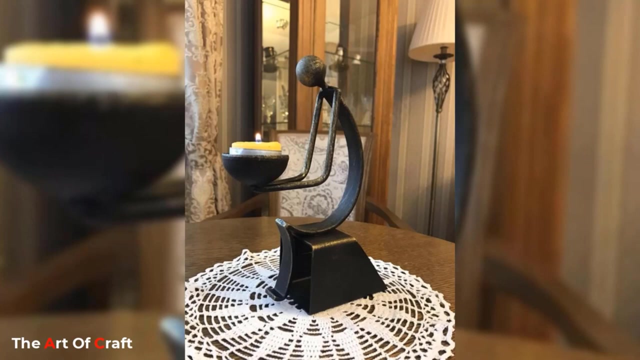 clear plan, the right tools and materials and a passion for creativity. So what are you waiting for? Get started on your first scrap metal project today. I hope you were inspired to watch these ideas till the end. Which one of these ideas was your favourite? 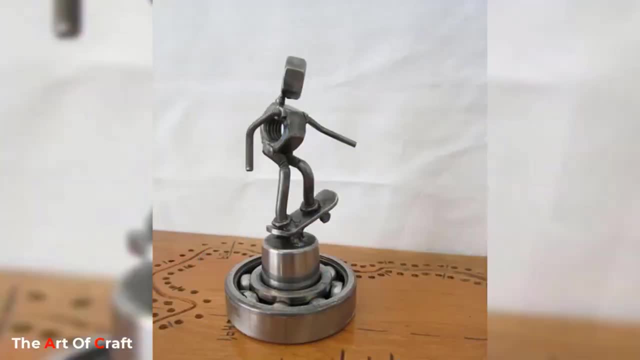 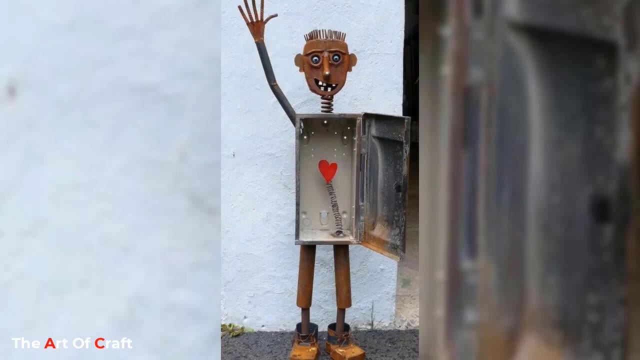 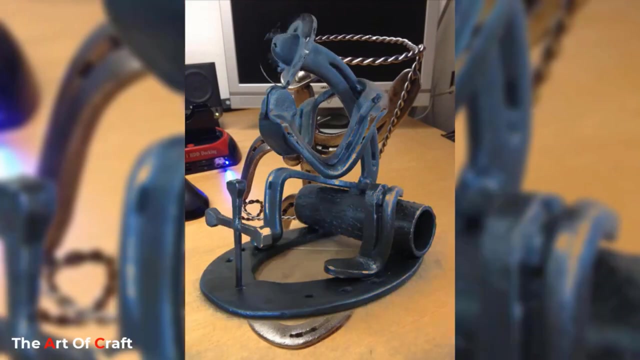 I'd love to hear from you in the comments If you'd like to keep up to date with my latest videos about DIY projects, woodworking, metalworking, furniture ideas and more. you can subscribe us and click the bell icon for notification when we upload a new video to the channel. 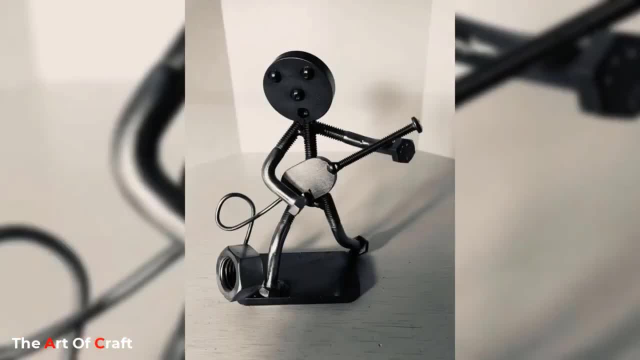 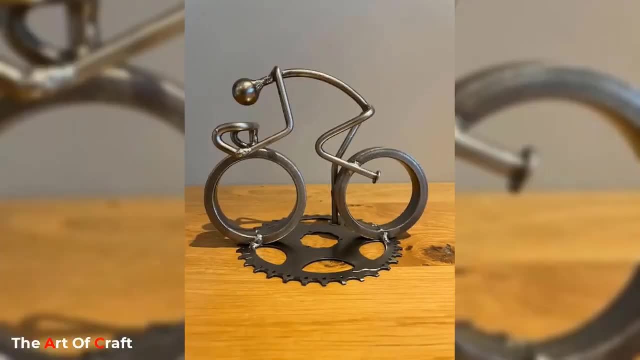 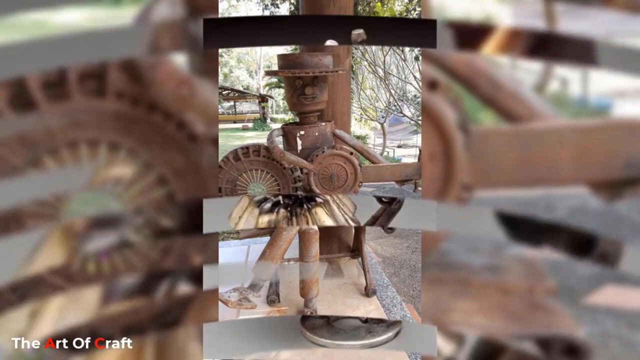 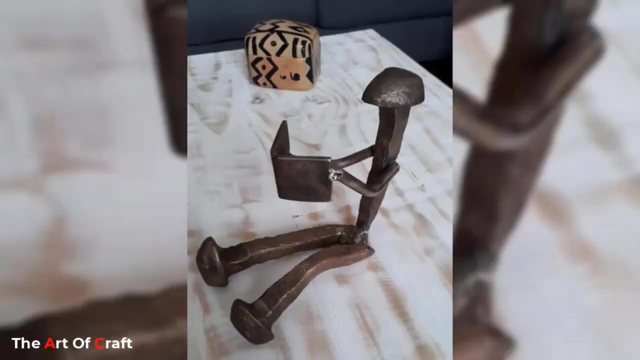 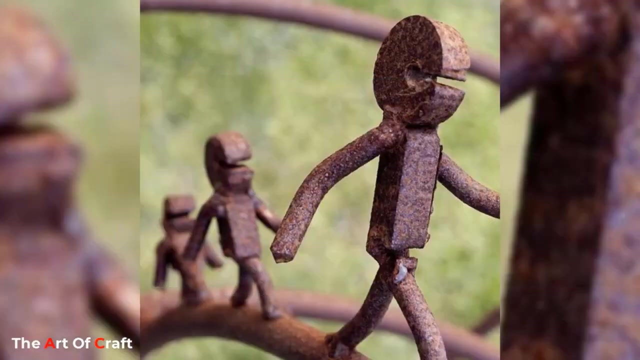 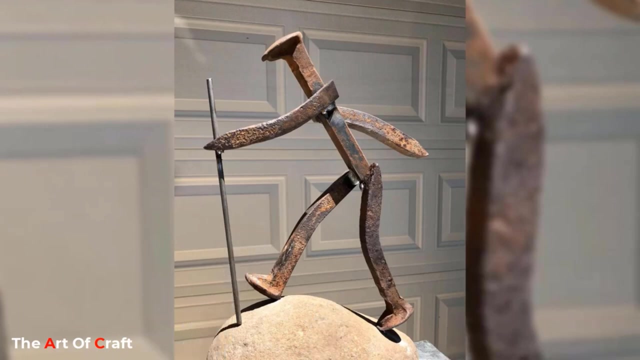 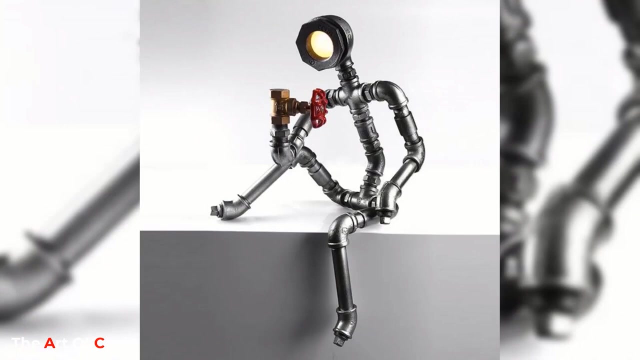 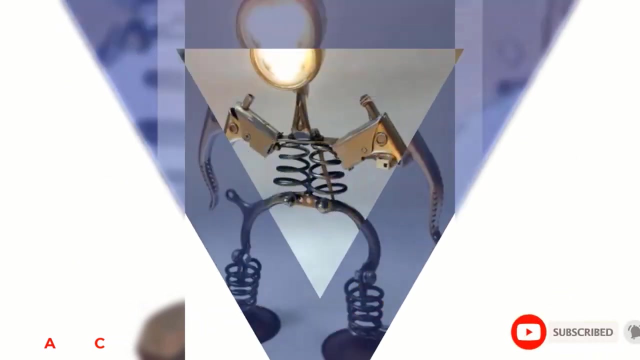 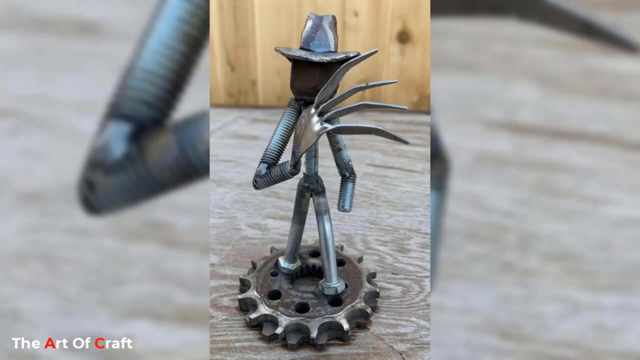 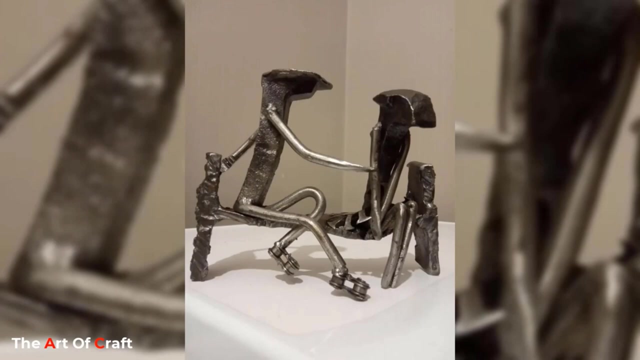 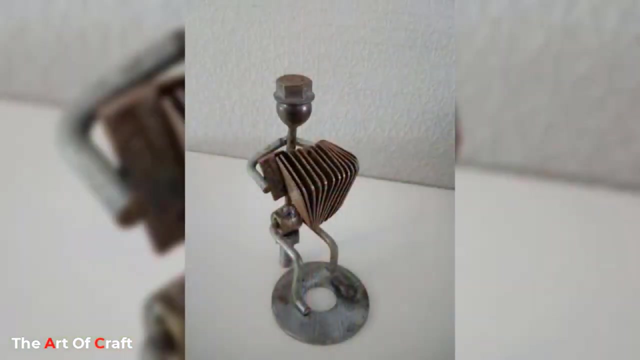 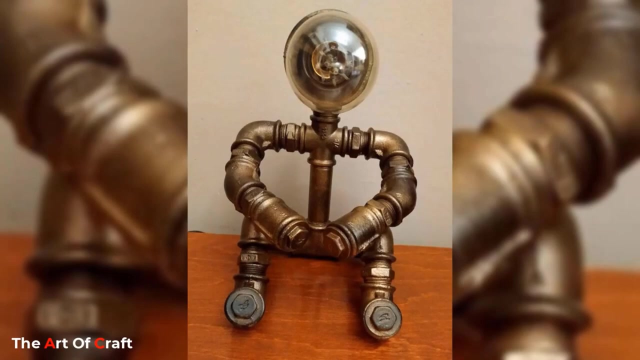 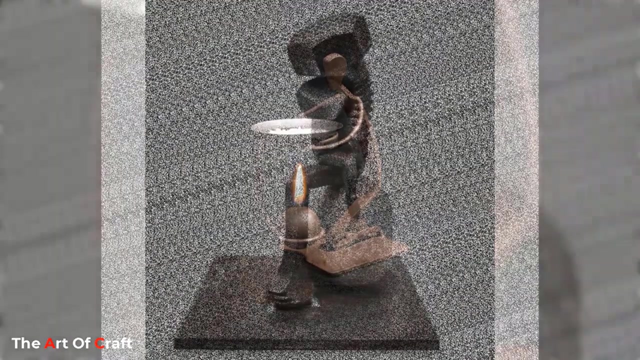 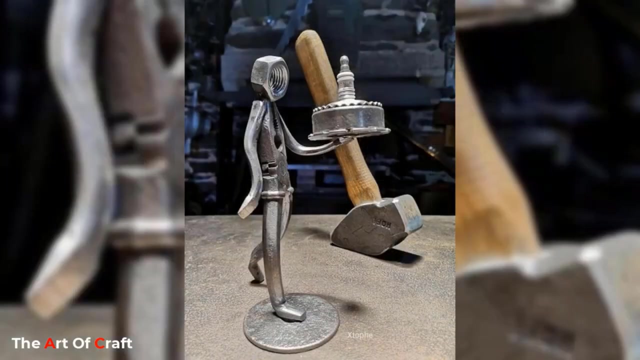 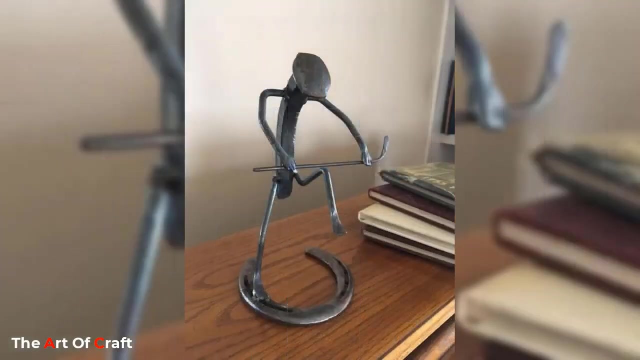 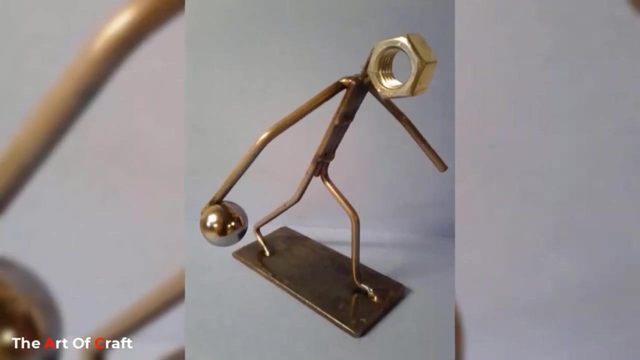 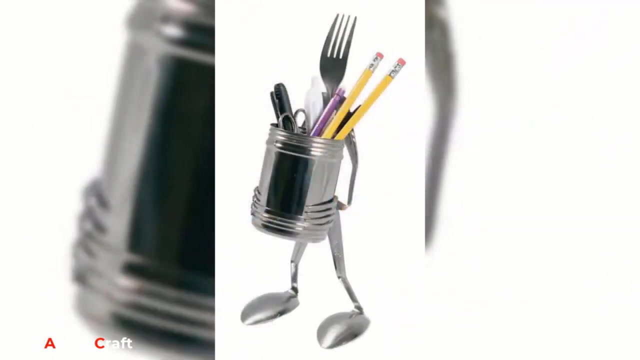 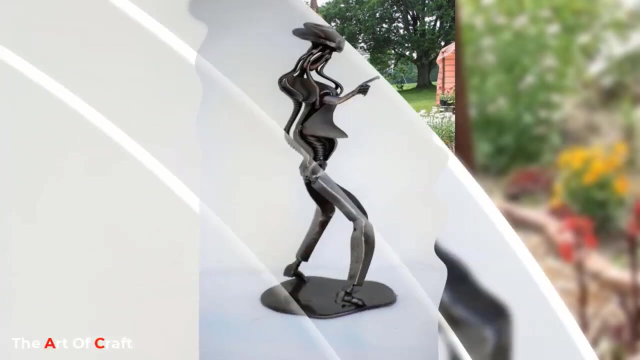 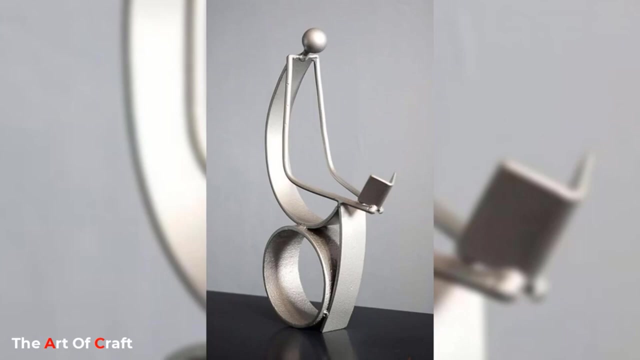 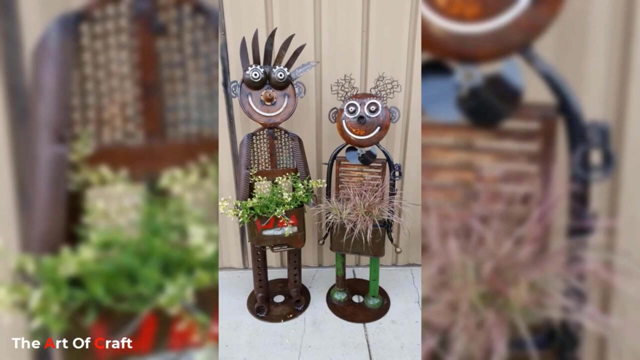 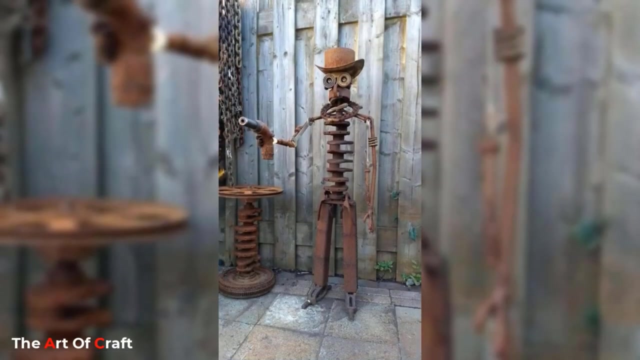 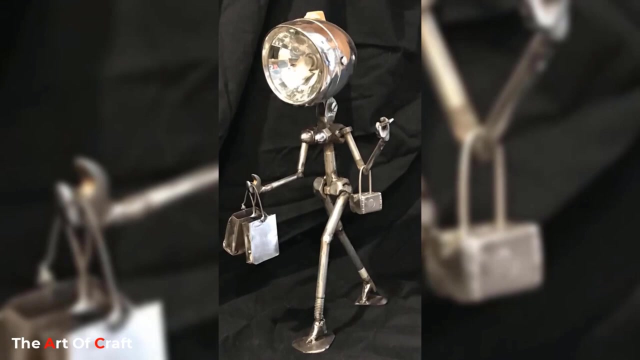 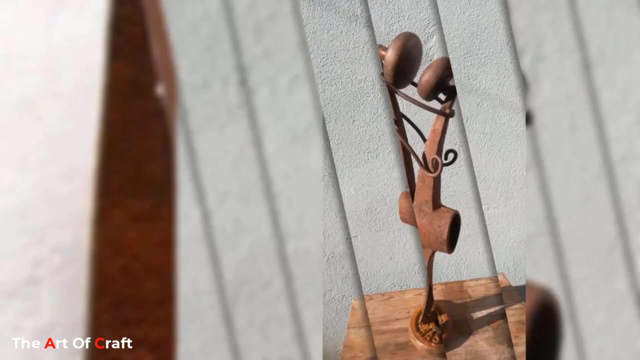 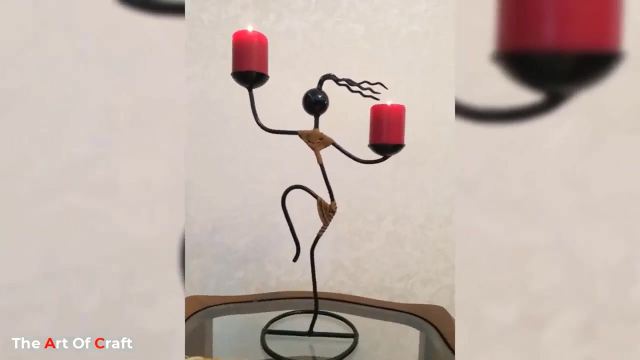 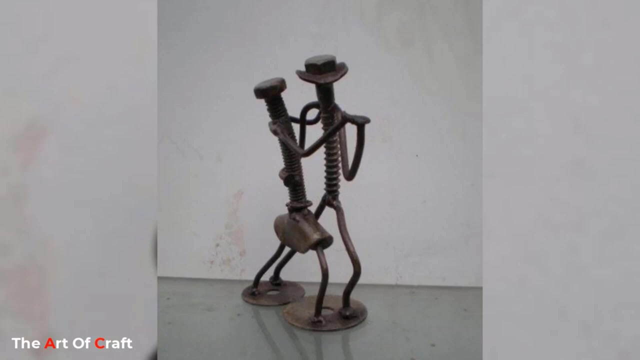 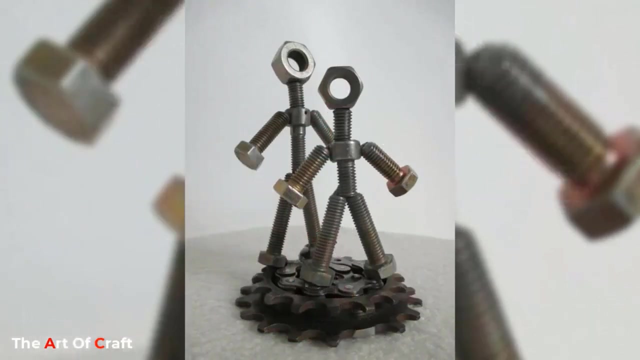 I'll see you in the next video. take care, bye-bye. Subtitles by the Amaraorg community- community. Subtitles by the Amaraorg community. Subtitles by the Amaraorg community- wwwamaraorg community. Subtitles by the Amaraorg community.